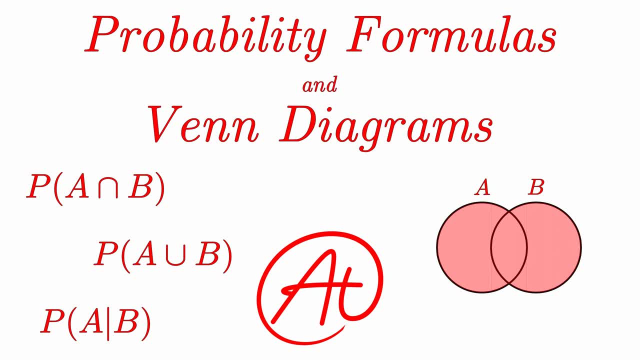 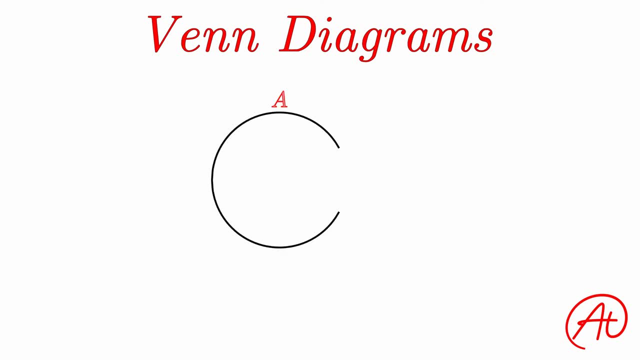 our channel to support us making these videos. Alright, let's dive in In your stat class. you've probably seen and may already understand how Venn diagrams work, but if not, they are essentially a way to visualize probability where each circle 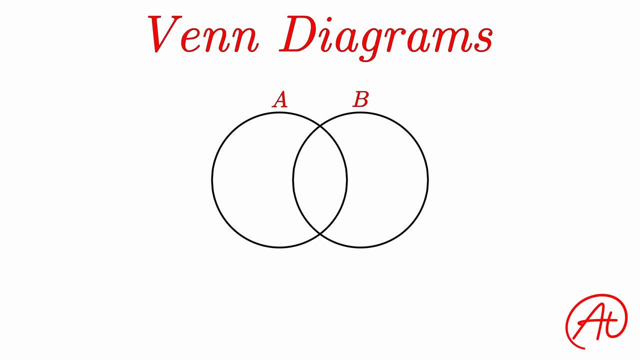 represents the probability of some event occurring. For example, this circle represents the probability of some event A occurring and this circle represents the probability of some different event B occurring. But then what about this overlapping region here? Well, this is one of the most common probability formulas I've ever used and I'm going to. 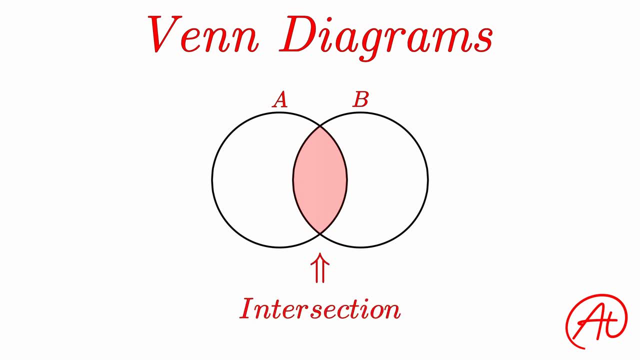 explain it to you. This is known as the intersection of A and B, written like this: Now, basically, what this region represents is the probability of both A and B occurring together. For example, if we were randomly selecting a playing card, we might have A be picking a jack. 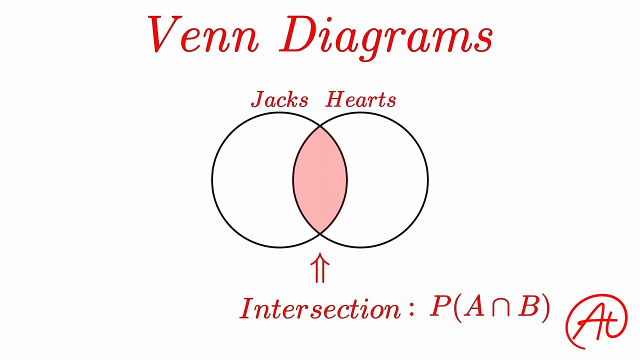 and B being picking a heart. In that case, in this left circle, we would have cards like the jack of diamonds, the jack of spades and the jack of clubs. In the right circle, we would have cards like the two of hearts, the three of hearts, the four of hearts. 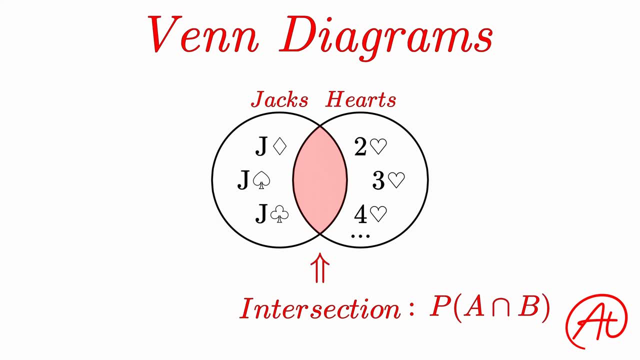 and so forth. However, there would only be one card that both circles share, and that would be the jack of hearts. So we place that in the intersection of both circles. Now that we've covered the intersection of A and B, we can go over the union of A and 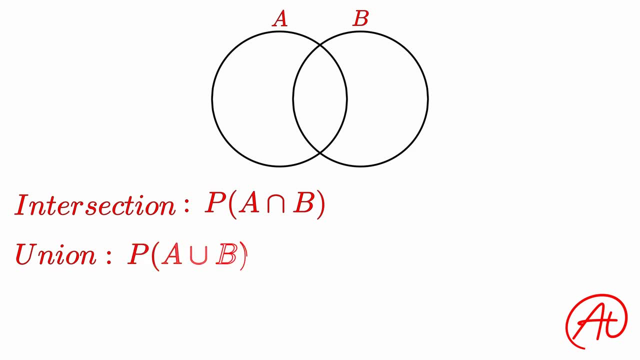 B. The union is written like this, which is read as the probability of A or B And, just like it's sounds, it represents the probability of A or B occurring. For our card example, this would mean that we are trying to find the probability of picking a jack that isn't a heart, a heart that 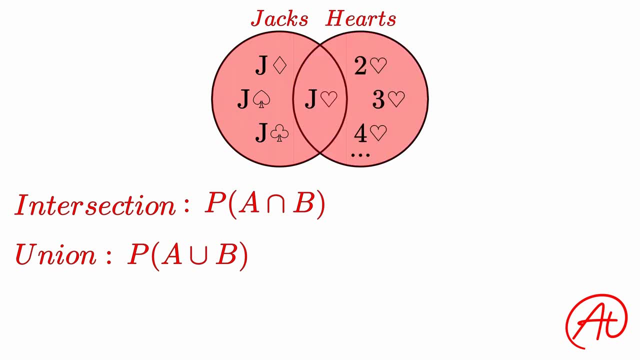 isn't a jack, or even a jack, that is also a heart, Essentially any area within the Venn diagram. Okay, but how do we calculate this value? Well, one way would be to take the entire probability of picking a jack and put it in the intersection of A and B, and then put it in the intersection of A.